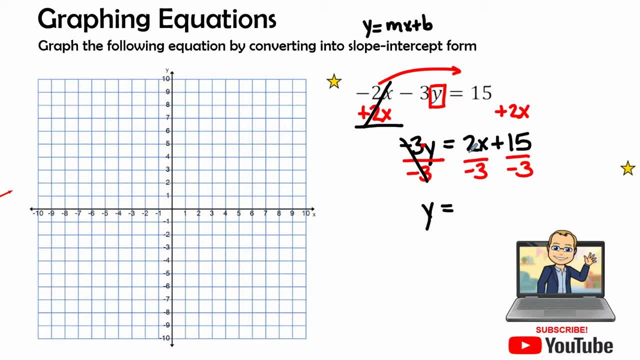 And then we divide two times out of this result and we get a negative 3 by a negative 3.. And then the big thing in the first matrix is the fact that 2x is two sixths and we're not proceeding through the whole matrix, So we're not proceeding through all PB, first wit, and then we have two. 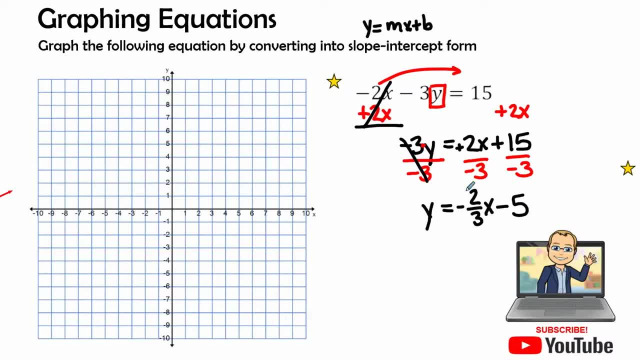 thirds, with a negative. It's like It's like. It's like we have our equation in the y equals mx plus b form, or what we know as the slope-intercept form, where we have our slope right here and then we have our intercept or our y-intercept. 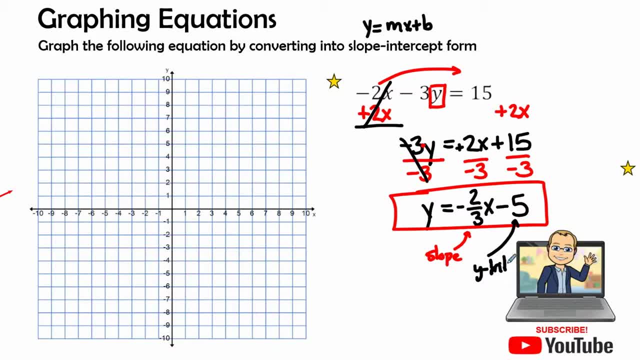 right here, right there. So the y-intercept is the number that we start with. So that's our starting point. We start at a negative 5.. So I start at my origin and go down to a negative 5, and then I'm going to build from there. So we look at our rise over our 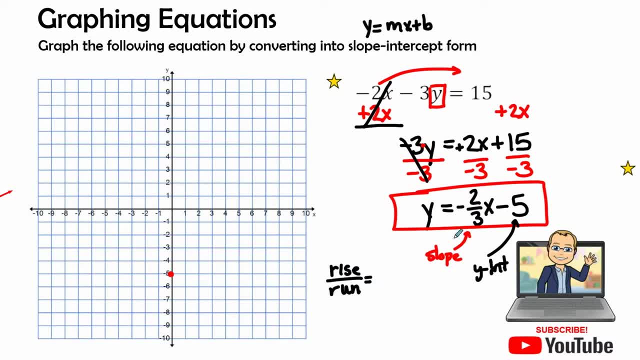 run. That is our slope And we see that we have a negative. 2 thirds That negative I'm going to put with a numerator. I could put it with a denominator, but I'm going to go ahead and put it with a numerator. 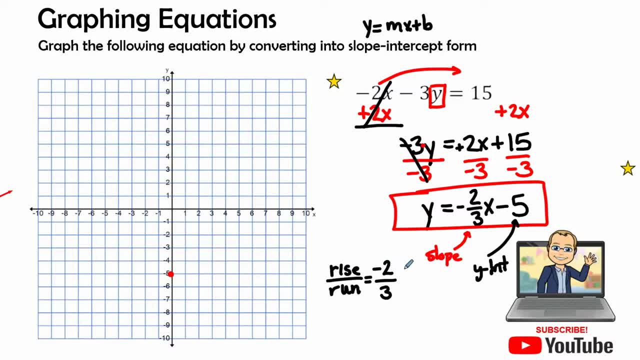 And this is going to tell me that my rise is a negative 2. That means I'm going to rise downward. That means I'm going to go in a negative direction. Rising is either up or down. rise up or down on the y-axis. And so the run is going to the right because it is. 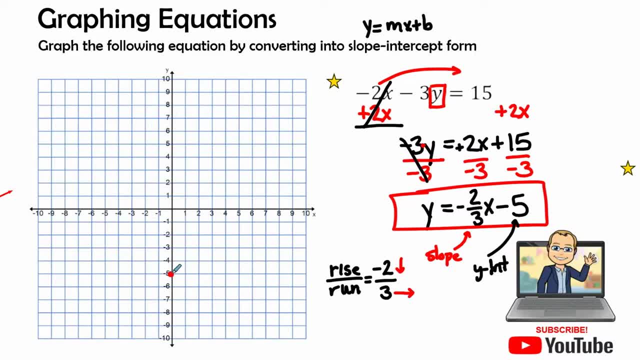 a positive number. So if we look at our starting point right here we are going to go down to our runners and there's our decline of negative 2 and we are going to move to the right to 3 for our next point on the coordinate graph. Now we just need two points, That's. 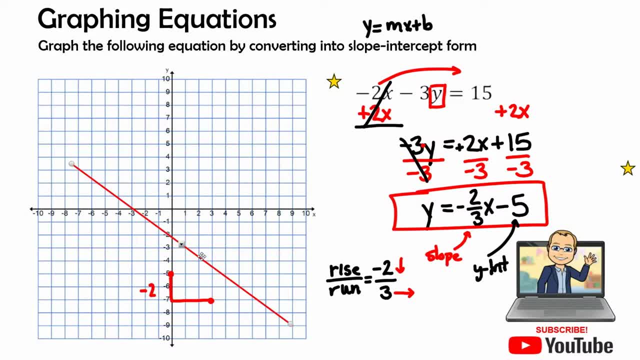 all we need to graph this line. So we're going to need two points and we can put them right there. And there we have The line for y equals negative two thirds X minus 5.. Okay, that was cool. Let's go ahead and try one more and let's get rid of this line. 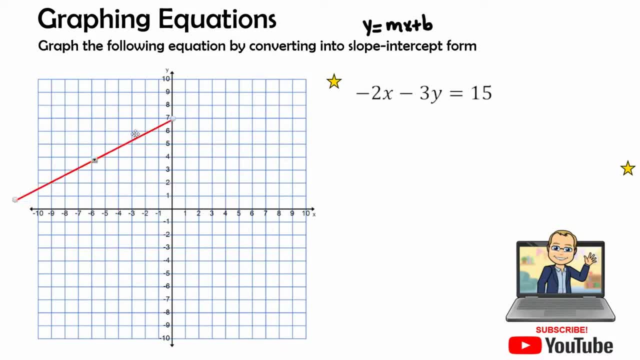 We're going to bring this line back, I guarantee you. So let's go ahead and move the standard form off to the side. Let's see what the next equation brings to us. The next equation is: x equals 2y minus 8.. Now, it's not necessarily in the slope-intercept form, so we're going to once. 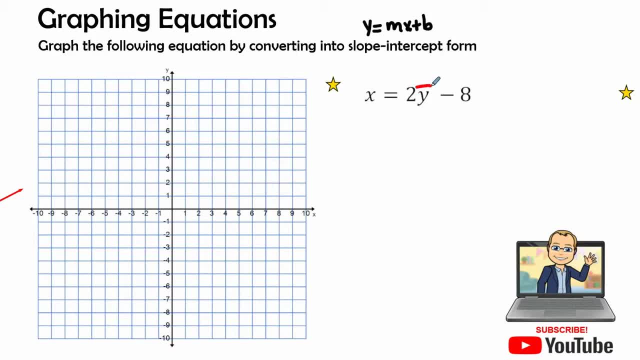 again isolate our variable y. We're going to isolate our variable y and move everything else onto the other side of the equation. So the inverse of a negative 8 is a positive 8.. There we go, and negative 8 plus 8 is 0, but I have to put it on the left-hand side as well. 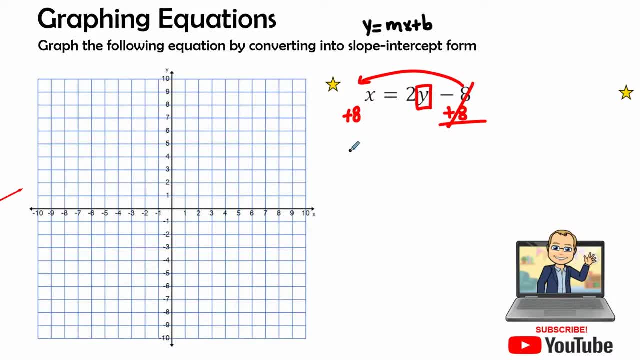 so we can balance our equation. So when I rewrite it I have x multiplied by 2y plus 3x minus 2y plus 3x minus 2y and I have to keep it on the left-hand side. 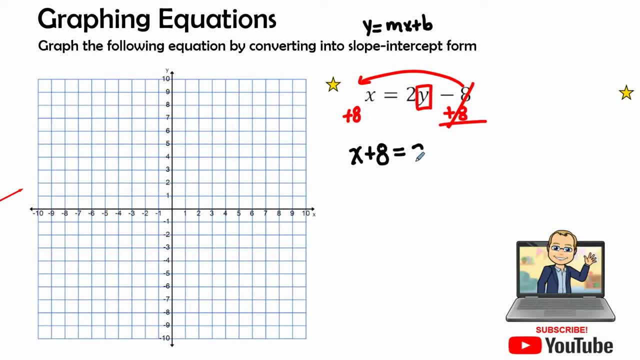 plus 8 equals 2y. Now, since it's an equal to each other, I can switch all the terms on either side around. So I can switch it around. So 2y equals x plus 8.. I have to make sure I keep this as a 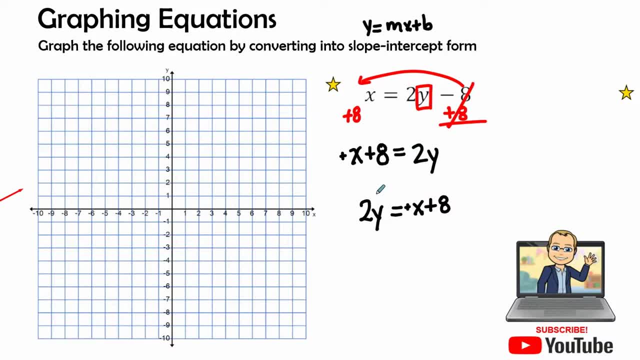 positive. So I need to make sure this stays a positive. This was a positive, And if it was a negative, I need to make sure I put the negatives in the right area. So right now we have: 2y equals x plus 8.. So that 2 is connected to the y by multiplication, And so we are going to divide by 2. 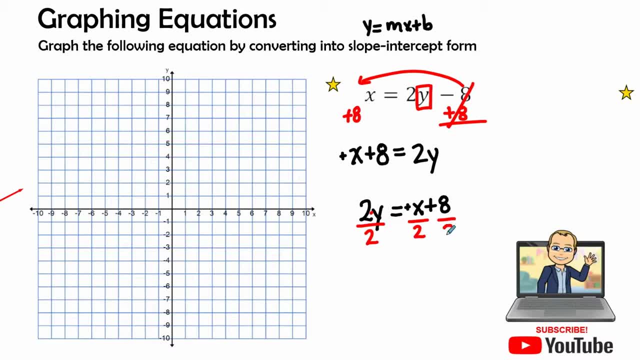 under each term. Therefore, this becomes 1 and we have 1y equals x over 2.. Wow, that x equals x over 2.. There is a coefficient or a number in front of that x And we say it's a imaginary 1.. It's a 1. 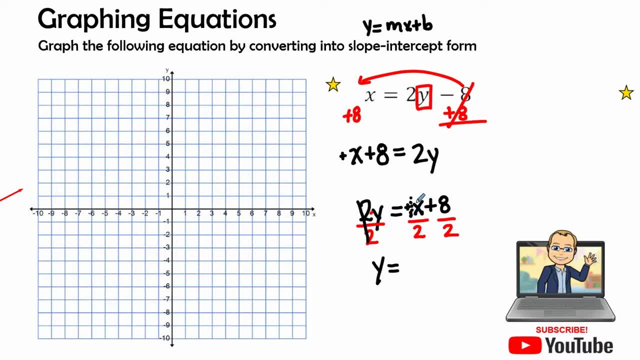 there It's a 1x, We just don't have to write the 1.. So that helps us find out what our slope is going to be. It's going to be a positive 1, half x, And then 8 divided by 2 is a positive 4..